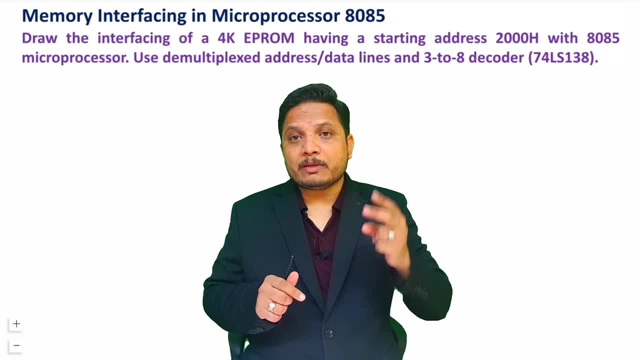 when we talk about RAM at that time there are two categories of control signals that we need to give from microprocessor to memory. Those two control signals are memory read as well as memory write And, very essential part that is cheap: select So whatever address and data that is. 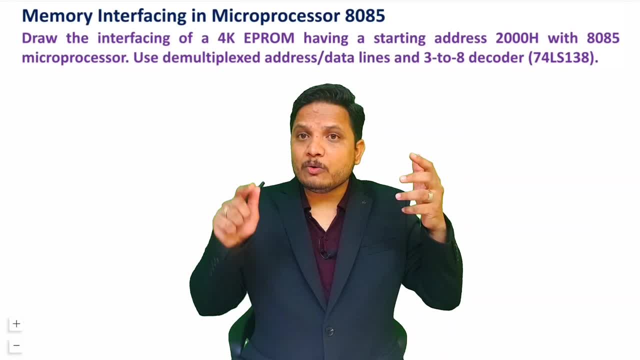 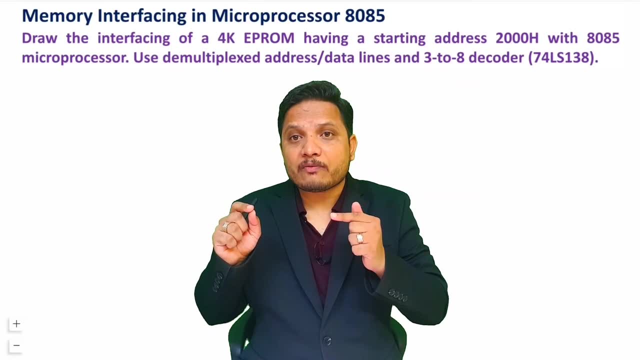 been given by microprocessor that should be given to well defined address and that will be only given if you provide decoding of that IC and that decoding will be given to respected chip select of IC. So there are basically four different types of signals that you will. 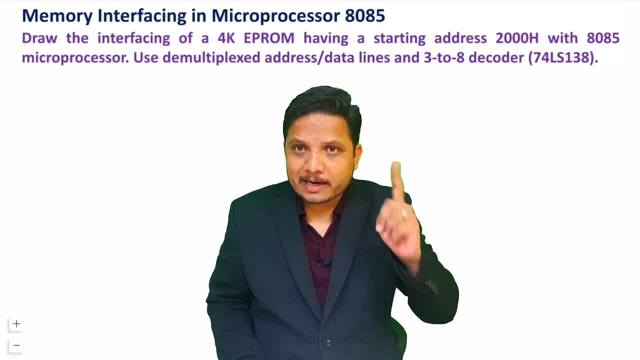 have to identify for memory interfacing address line, data line, control signal and chip select. So how to do that entire process that I'll be going to explain you Right. So there will be at least three, four examples that you will have to watch it from this platform so that you will be able to. 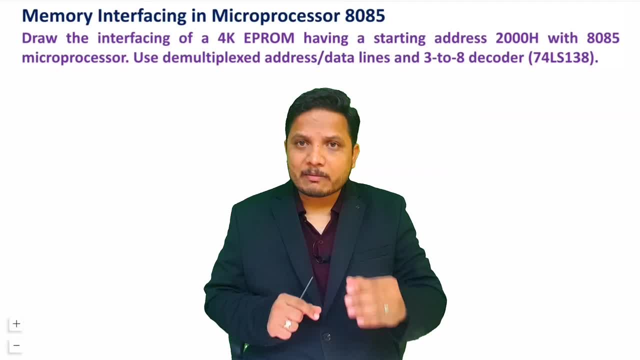 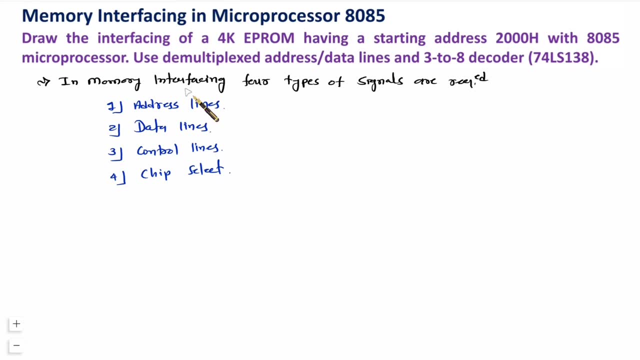 explain any equation, So let me write that first. So, my dear students, in memory interfacing these four categories of signals that we need to identify. So, first of all, address lines and data lines that we can identify based on size of memory and control signal that we can identify based on which type of memory is given to. 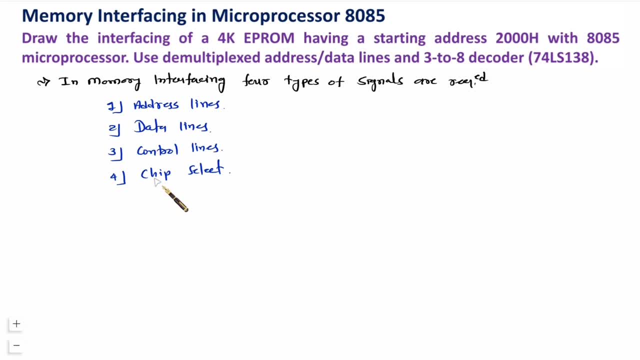 you And at last I'll explain you how to identify chip select Right. So, my dear students here in question, draw the interfacing of 4k EEPROM having a starting address. 2,000 hacks with 8085 microprocessor, use demultiplexed. 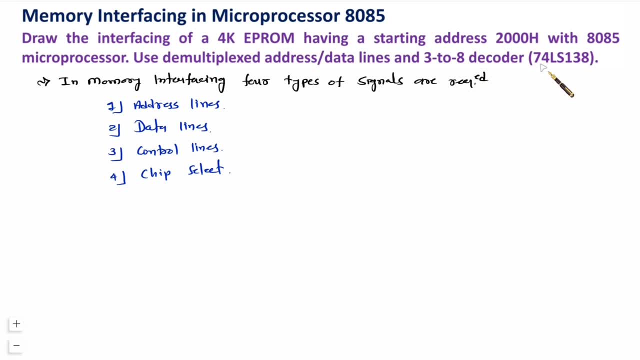 address, data lines and 328 decoder that is having number 74LS138. So first of all, I need to identify address lines and data lines. So here, my dear students, we have been given with 4 KB of EEPROM, right. With 4 KB of EEPROM, my dear students, we are having how many address lines? 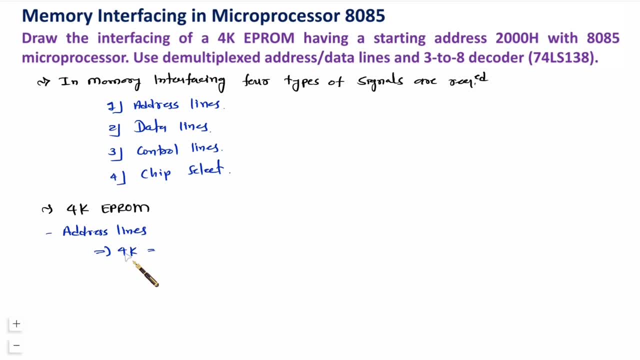 With 4 KB. what it means 4? K means 4 into K. What is the meaning of 4?? In terms of 2 to the power, it will be 2, and K means 2 to the power 10, right, So 2 to the power 12, that is how. 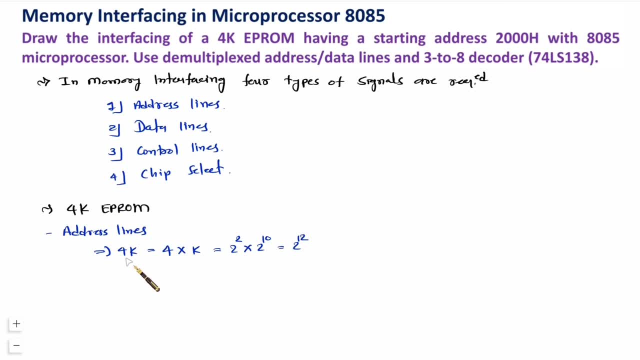 total data is there with 4 K. So, my dear students, 2 to the power 12 means here total 12 address lines are required And here 4 K EEPROM. that is having 8 data lines, And you see. 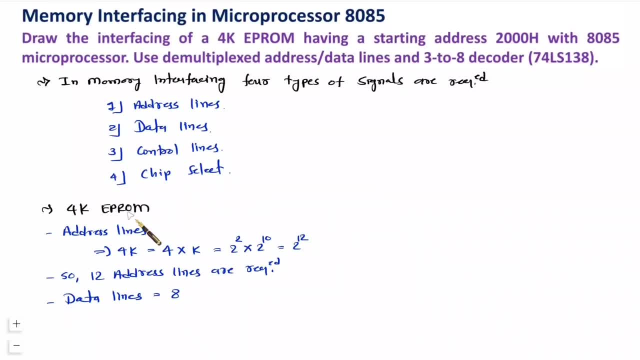 it is erasable, programmable ROM, right. So, as it is ROM, here we need to interface memory read terminal with ROM, right. So control signal that will be memory read only. Now, my dear students, here we have identified address lines, data lines, 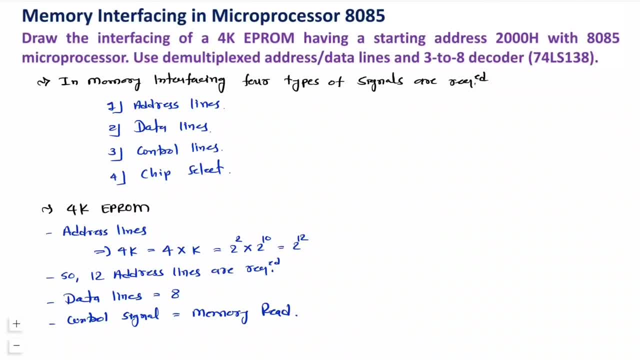 control signals right. So now we need to identify chip select and chip select that we can identify based on memory map. So you see here 4 K EEPROM that is there with us and its starting address is 2000 hex. So how to have memory map. Let us try to understand that. 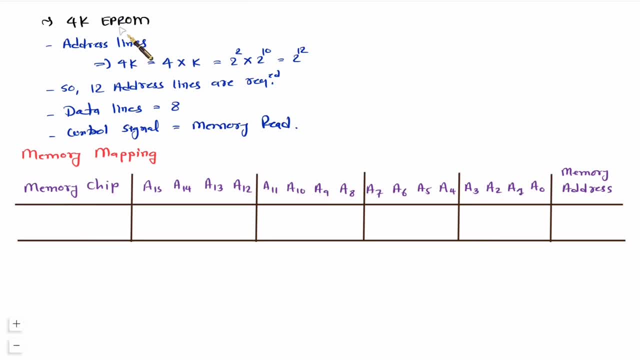 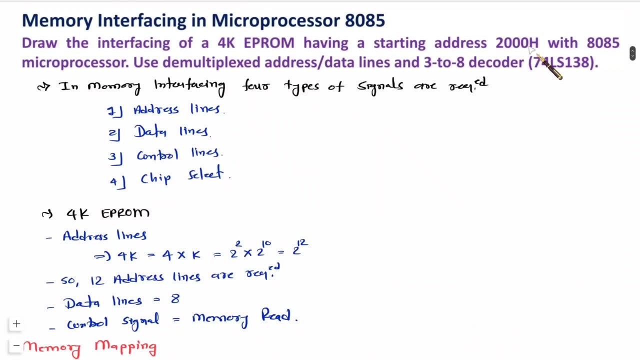 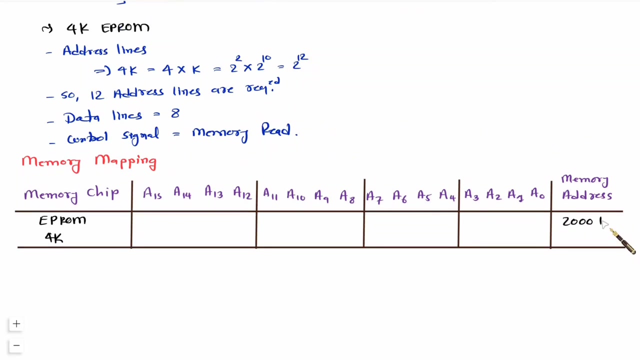 So, my dear students, here, memory chip that is given to us, that is EEPROM with 4 K. So here I am writing, EEPROM with 4 K. memory chip is there and starting address that is given in question. you see that is 2000 hex. So here I am writing 2000 hex. That is my starting address. Now, my dear students, 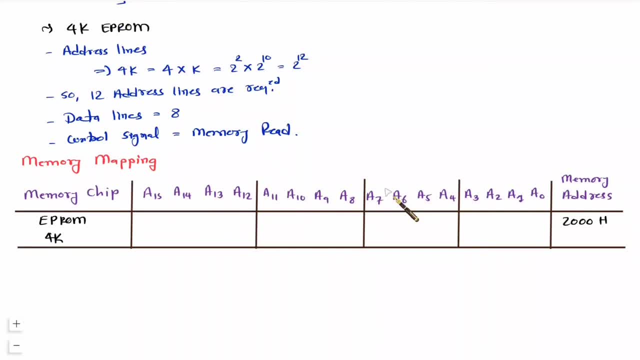 here with 8085, we have total data. So here we have total data. So here we have total data. So 15 address lines a, 0 to a, 15.. So let us write this in terms of bits. So you see I have bisected. 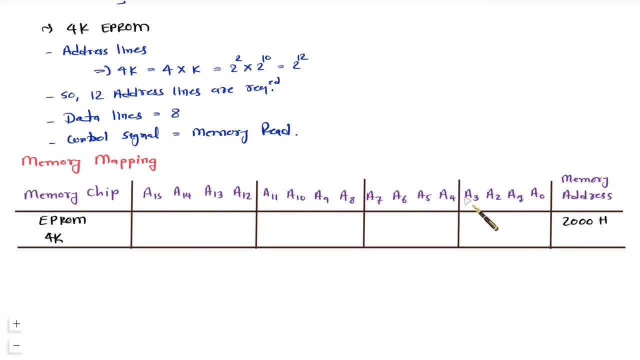 this in 4, 4 bits, as it is there in terms of nibble, and you can easily write it from hexadecimal address. You see, 0 means 4: 0s are there. Then again, 0 means again 4: 0s are there. 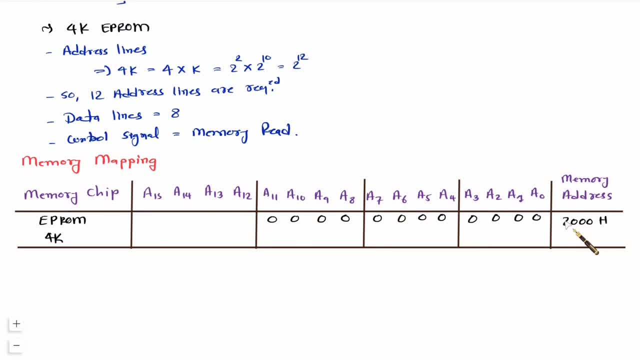 Again. 0 means again 4 0s are there And then 2 means 0010.. That is how starting address that identified. now you see, address lines are how many address lines are 12, right? so 12 address lines that you should be using it from a 0 onwards, right? so here i'll be using it from a 0 to a 11. 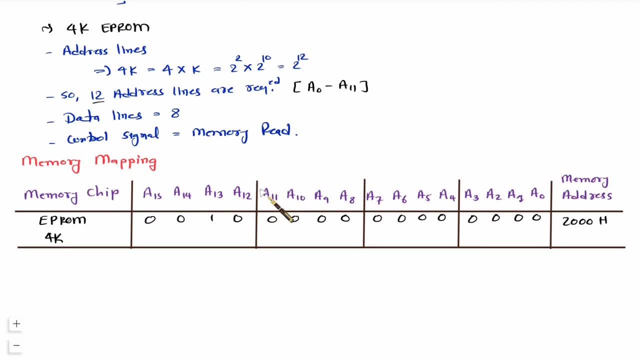 right. so a 0 to a 11 that you need to focus about and from 0 to 1 you will have to give transition means this much amount of memory that we will be using right. so you see, those are getting 1 from 0 right and these are the lines which we are not using it for address purpose that we will. 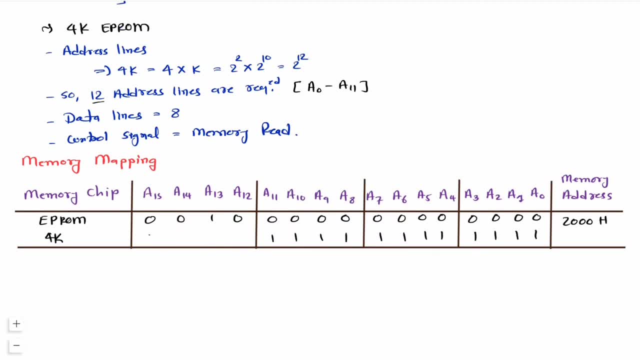 be using it for chip select and that will stay as it is. so you see that is 0 0, 1 0. so now we need to write address in terms of hacks here. so you see this is 0 0, 1, 0 means it is. 2 0 1 0. so now we need to write address in terms of hacks here. so you see, this is 0 0 1 0 means it is 2 0 1 0. so now we need to write address in terms of hacks here. so you see, this is 0 0 1 0 means it is. 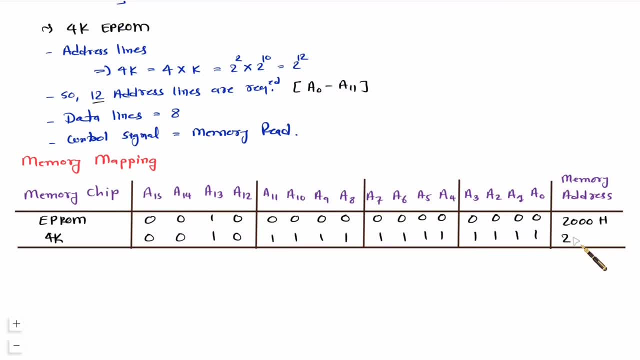 2 0, 1, 0. so now we need to write address in terms of hacks here. so you see this is 0, 0, 1, 0 means it is 2 and these are ones right. so these are all. once means f, f, f, so starting address, that will be there. 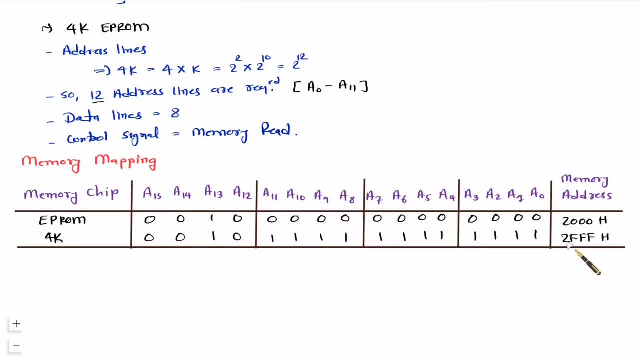 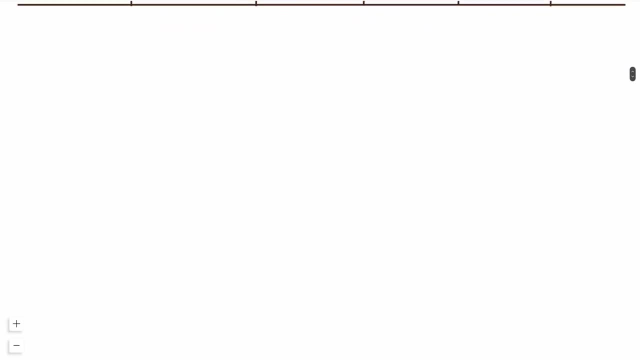 with 2000, as per the equation, but ending address, that will be 2 f, f, f with 4k of epirom. now, my dear students, i'll explain you how to have memory interfacing. so for that, my dear students, what i'll be doing is i'll be taking microprocessor 8085. 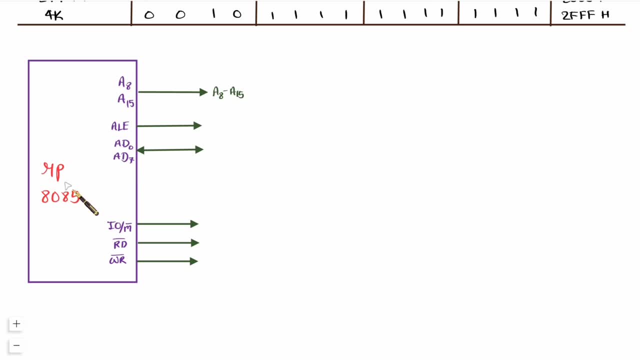 microprocessor 8085 over here now, my dear students, if you observe, with microprocessor 8085, address data line, those are time multiplexed and that is bi-directional. here we will be using address latch. enable to latch address from this, ad0 to ad7 and a8 to a15. those are address lines only and here to generate. 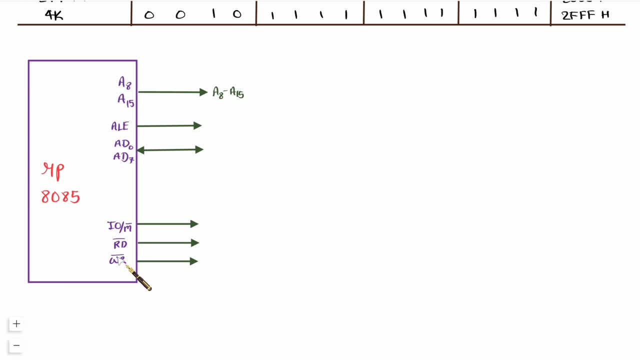 control signals. we have io memory bar, read bar and write bar right now. first of all, i'll explain you how to demultiplex this address and data right. so for that we need to have latch. so, my students, you see i'm using one latch over here, that is 74 ls 373, what it will do here we have. 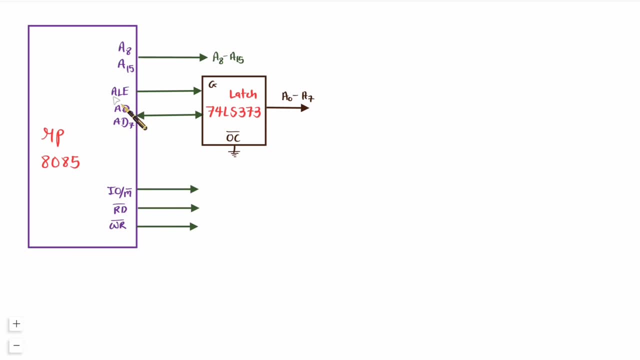 g terminal, that is enable terminal, to which we will be connecting ale. so whenever address latch enable is given over here, it will latch address over here, and here we have data right. so you will be using this data, that is d0 to d7. now, my dear students, here we are delivered. 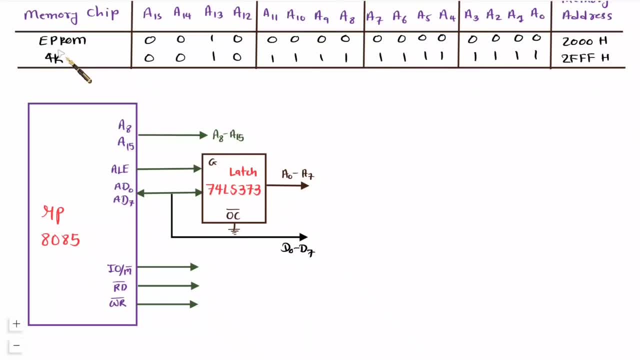 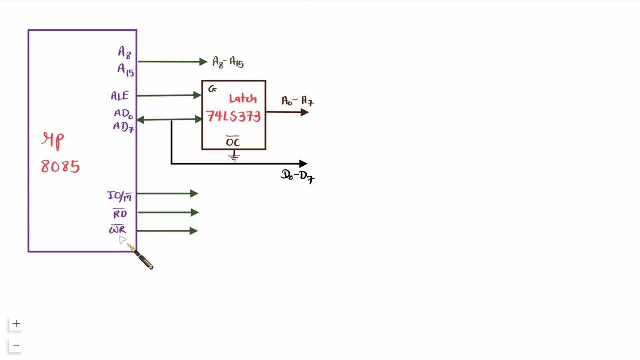 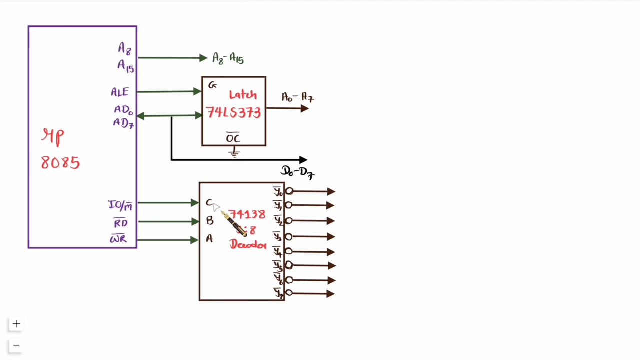 to interface ep rom. so for ep rom control signal that should be memory read. so here see, we have io memory bar, read bar and write bar. so based on this we should be generating control signals right. so by using 3 cross 8 decoder, i'll be using it. so you see io memory bar that is connected with c, this read bar, that is. 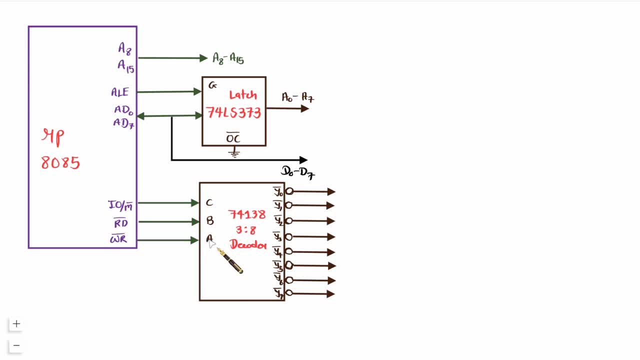 connected with b and write bar that is connected with a. so here we have decoder that is having three inputs- a, b, c. if i write it over here- a, b, c- then, my dear students, based on the value, it will be selecting output lines, right. so now you see, what we will be doing is we will be using this. 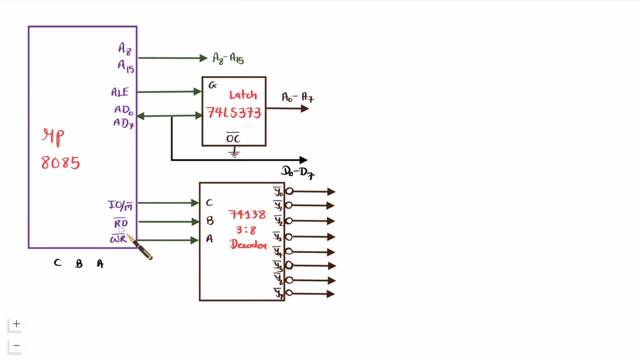 we will be generating memory read signal. so how to generate memory read signal here? io memory bar- that should be zero, here, read bar that should be zero and write bar- that should be one that will generate memory read signal. now, as if it is zero, zero one. it means that zero, zero one means y1 will. 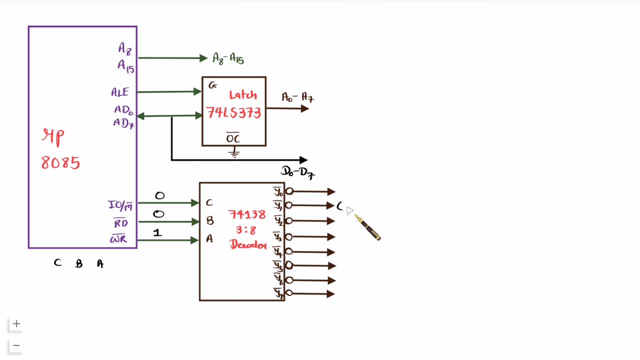 get selected so active low y1 signal, that will be our memory read signal and we will be generating read bar signal over here right. similarly, as if you wanted to have write bar signal, then what you need to have for write bar signal, my dear students, io memory bar, that should be zero, this read bar. 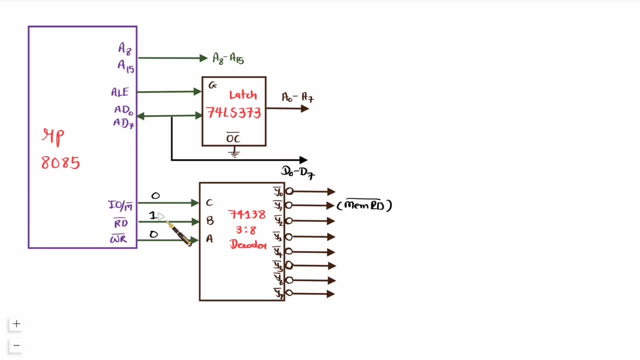 that should be one and write bar that should be zero. so zero, one, zero. what it means it is two. so y2. that will be memory write bar signal and we will be generating memory read signal over here. so we will be generating memory read signal over here. this read bar will be the same as usull read. 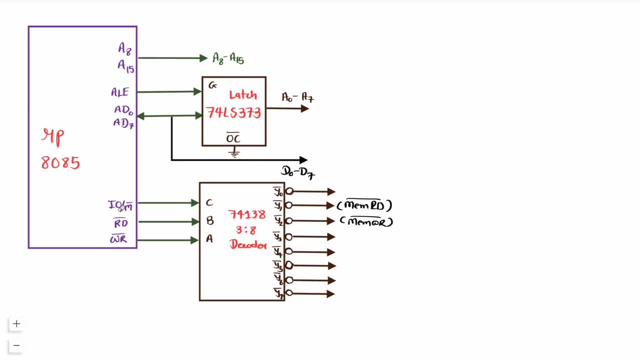 signal, right. similarly, as if you wanted to have io read, then this io memory bar, that should be one, and read bar that should be zero, and write bar that should be one. so one, zero one means it will be phi, right, so wi-fi, that will be io read bar. and as if you want to write io, in that case, here you will. 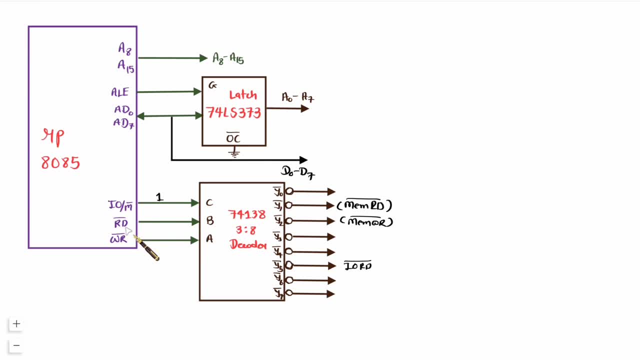 writing 1 for IO. then you wanted to have write operation, so read should be 1 and write should be 0, so 1, 1, 0 means 6, so y 6. that will generate IO write bar signal. so that is how we can generate. 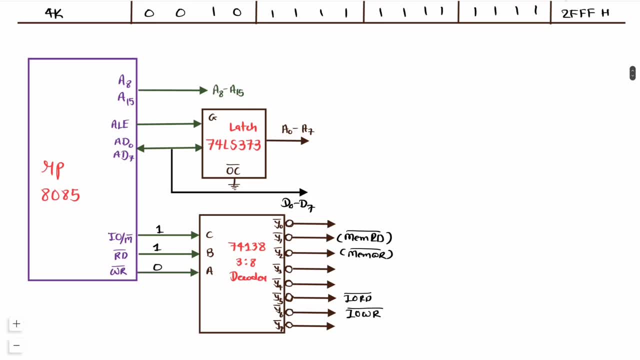 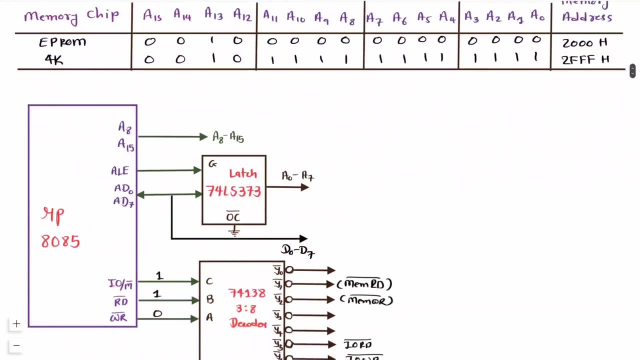 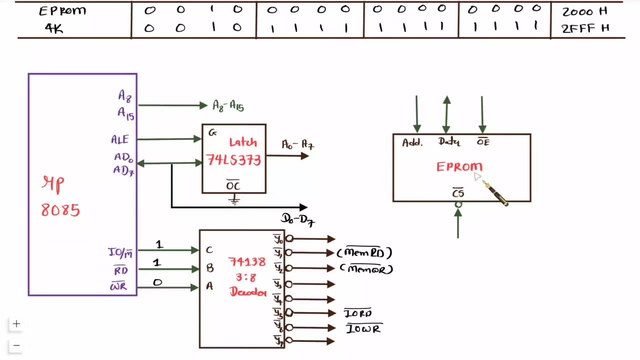 control signals. right, but for our case, my dear students, here we will be interfacing EEPROM of 4k and we need just memory read. so I'll be using memory read only now let me take that EEPROM. so, my dear students, here we have EEPROM and its size, that is there with 4k. so with 4k, how many address? 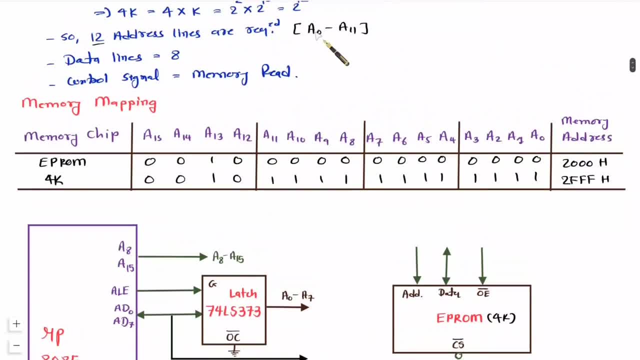 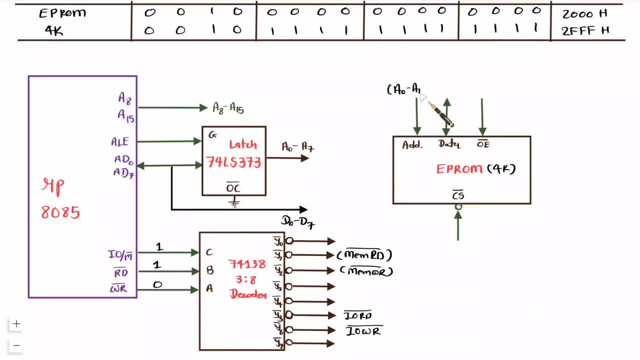 lines are there. address lines are there from a 0 to a 11. so here let me write addresses. that is there from a 0 to a 11, and you see that is going inside over here 4k and we need just memory read. so I'll be using memory read only now. let me take that EEPROM. so 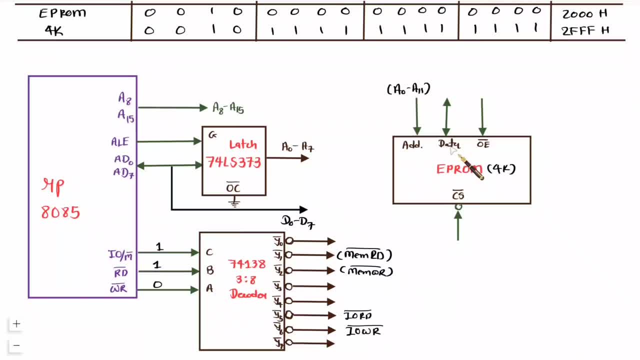 that is generated by microprocessor here data that is there from d0 to d7 and you see, here OE bar is there. OE bar means output enable. so memory read signal which we generated by this decoder that we will be connecting it over here, right? so what is memory read, this y1 bar of? 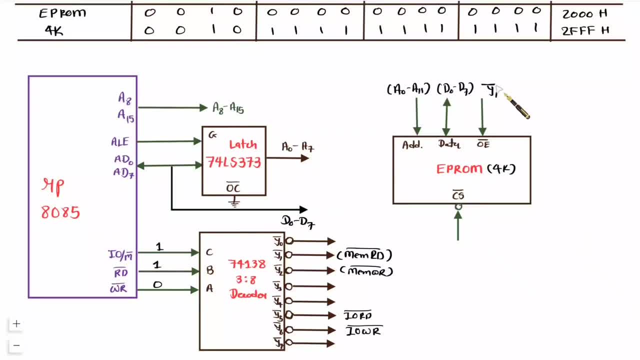 decoder. so I'm writing y1 bar here, right? so whenever you provide memory read output enable bar, that is there with EEPROM so you should not write memory read over here. it is output enable means when you ask memory read at the time, this EEPROM will enable out over here, right? 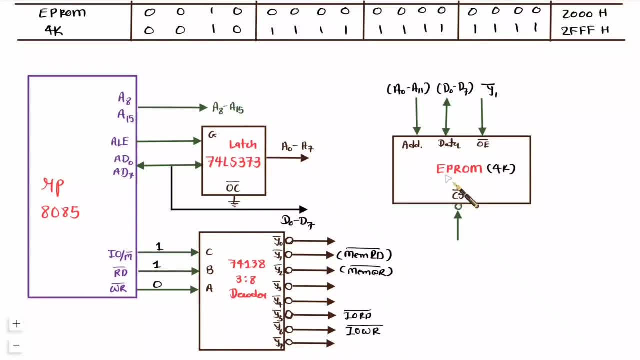 so this is output enable, which is there with EEPROM. now question is how to have chip select. so, my dear students, for chip select you will have to see what are the unused line. so you see a is in the line and b is in the line. so you see a is in the line and b is in the line and b is in. 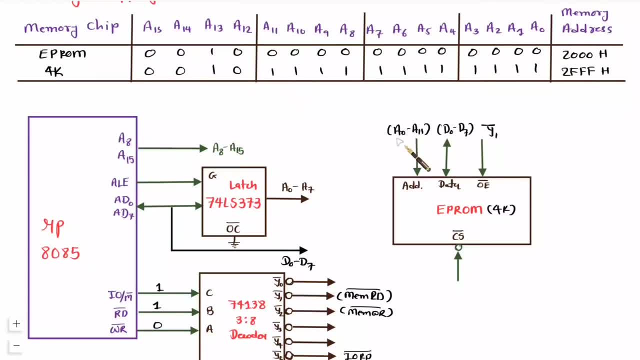 the line those are used for address purpose. now these are unused line that we need to see it for chip select and you see a 15 that is 0, 0, a 14 that is also 0, 0 and a 13 that is 1 and a 12 that is. 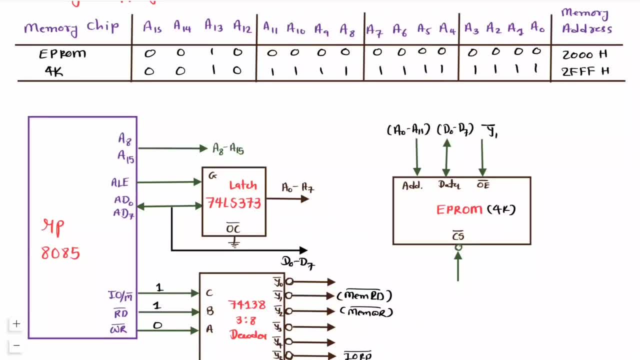 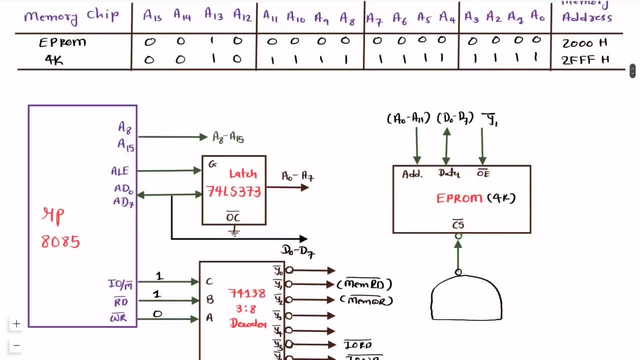 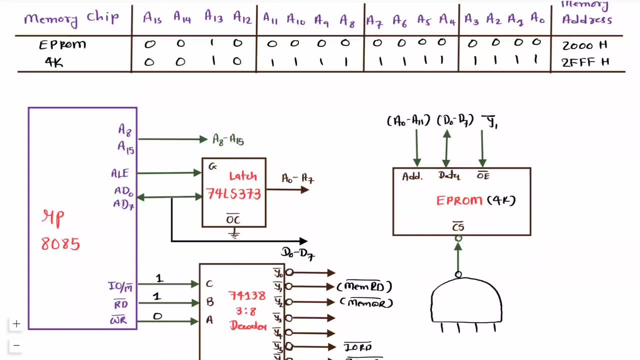 0, so how to use that for chip select. so you see, here you should be connecting one NAND gate. now here, my dear students, I have connected one NAND gate and you see, I'll be providing four inputs to it. now, you see, a 15 is 0. so what I need to do, by connecting one, 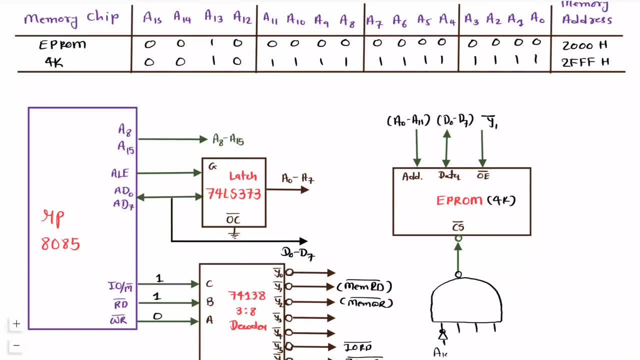 inverter, I'll be connecting a 15 over here. a 14 is also 0, so I'll be connecting it over here by connecting inverter right. so a 14 after inverter. now you see a 13 that is 1, so a 13 that I'll be. 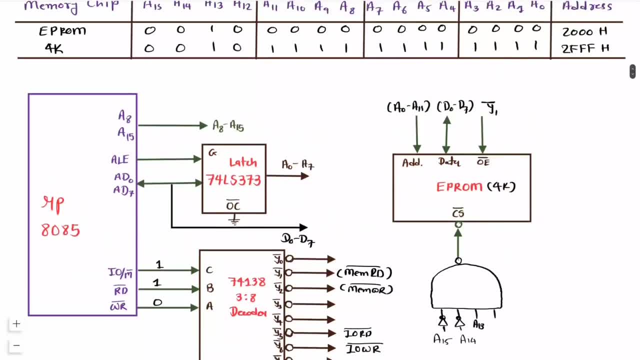 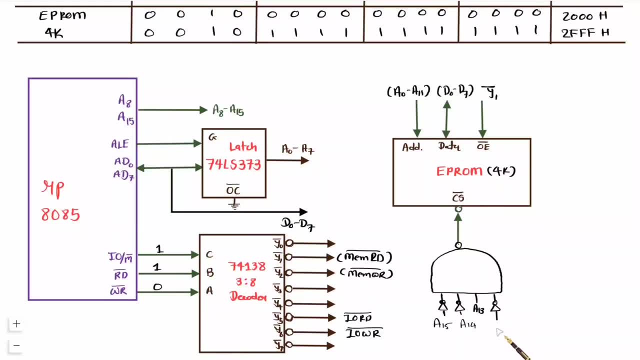 connecting directly over here and with this you see a 12 that is 1 and a 12 that is 1 and a 12 that is 0. so here I need to connect a 12 after inverter. so all the lines that I have connected here, which 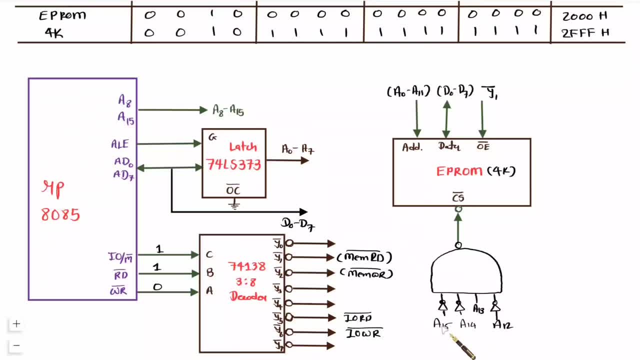 are unused and this chip will get selected only if this is 0, 0, 1, 0 right. otherwise this chip will not get selected and as if this chip is not getting selected, you cannot have address and data operation here. so what we are doing is we are providing unused line for chip select. it is, sir. 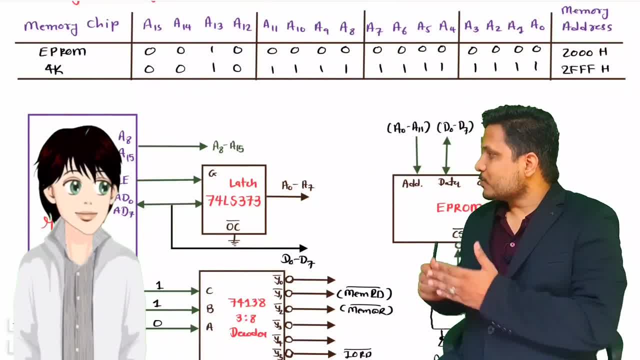 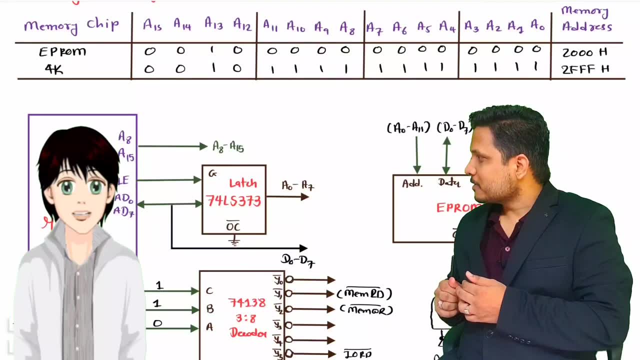 may I ask you one question? yes, definitely, John, you should ask me questions. I am here to reply your questions only. it is, sir, why you are using all the unused address lines. see, John, whenever we interface I see, and if you don't connect all the address lines with I see, you will not be able. 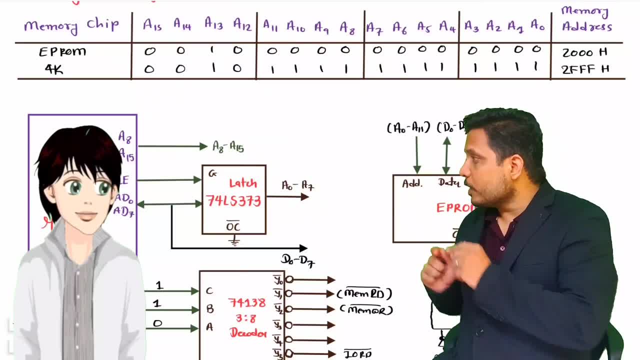 to use this chip select line right now. you can see here that the address line is not being selected. it is only being selected by the chip select line. so if I want to use this chip select line, then I have to use this chip select line. that is referred to here as partial decoding, see here. 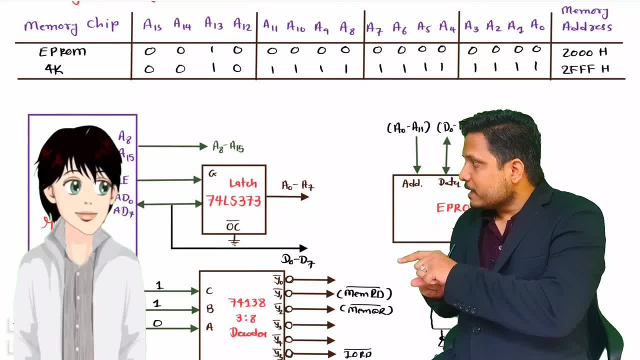 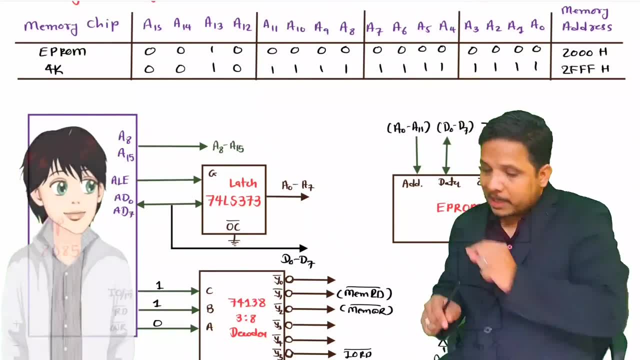 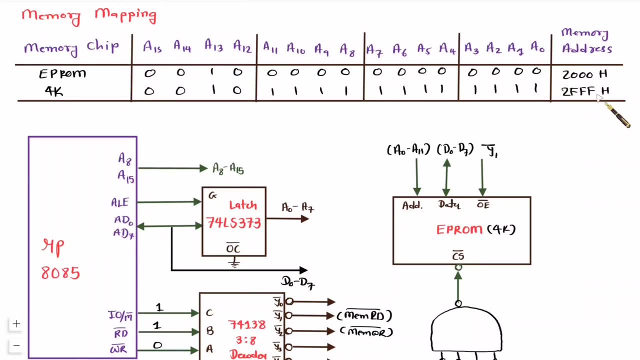 what we do is we decode that, I see, by chip select. if you don't use any single line for that chip select, in that case there is a possibility that false address may select your. I see, right, like you, hex, right now, these are the lines that we are using. let us say you don't use these lines, while 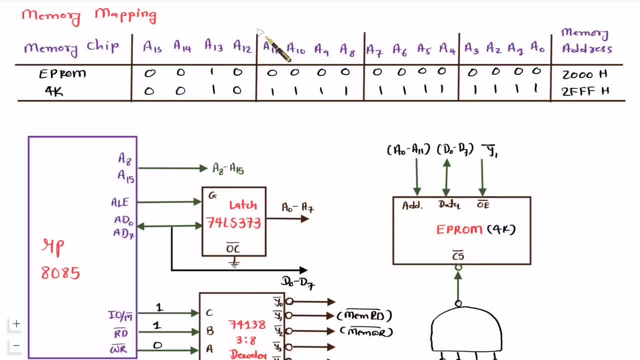 you have chip select over here. so what will happen? you will be using this only, so it is possible that for any random number over here, you will be selecting this chip and you may be accessing some data over here. so you don't want to access this data for other address addresses other than 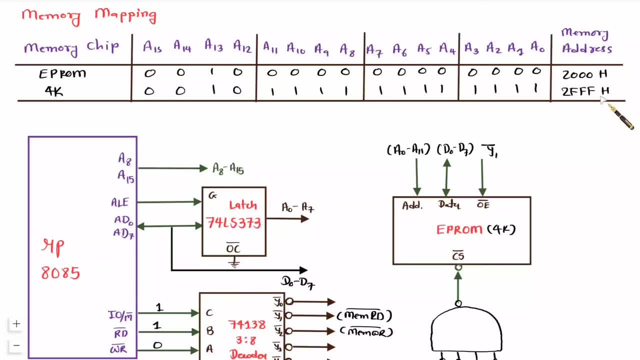 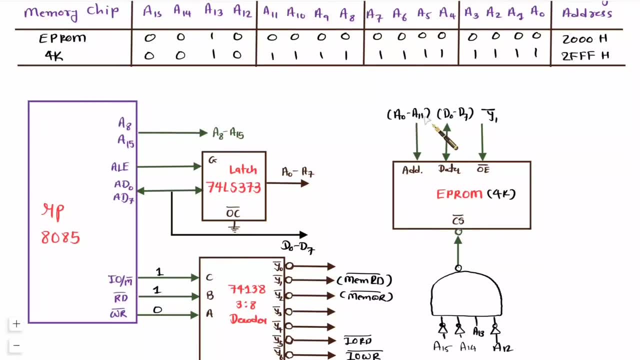 2000 hacks to 2 FFF hacks, right. so that is why you should be providing full decoding. this is full decoding. you see A 0 to 11 that is been used over here and A 12, A 13, A, 14, A, 15 that I. 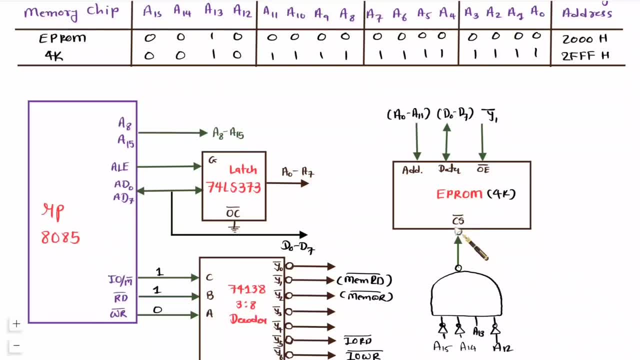 have provided here with chip select and I have not used decoder over here. why? the reason is this is just a single IC, so for interfacing of 1 or 2 IC we should not use decoder. the reason is this lockout gate of NAND gate that is easily available in the market with four inputs. right, and this is 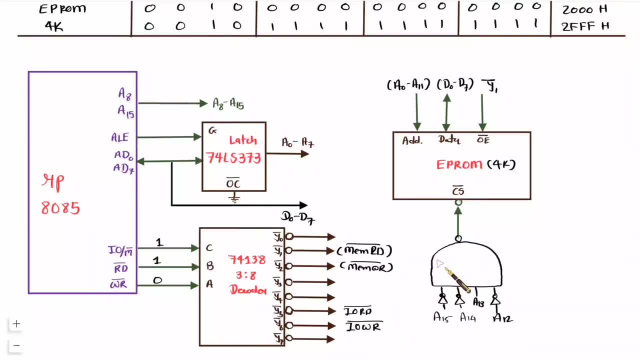 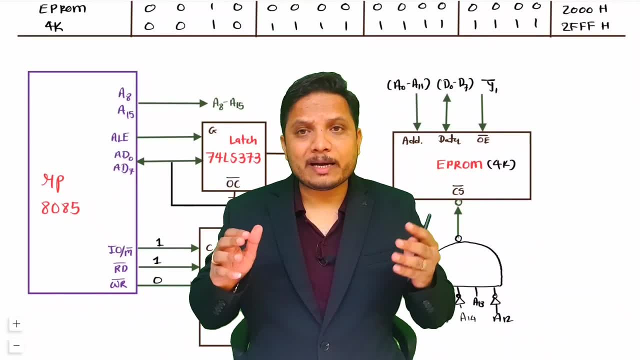 costlier IC compared to NAND gate. that's why you should be using NAND gate to have cheap, select four single or two ICs, right? so I think now, my dear students, it is clear to you how we should be interfacing IC. there will be three, four questions over here on this channel with this. 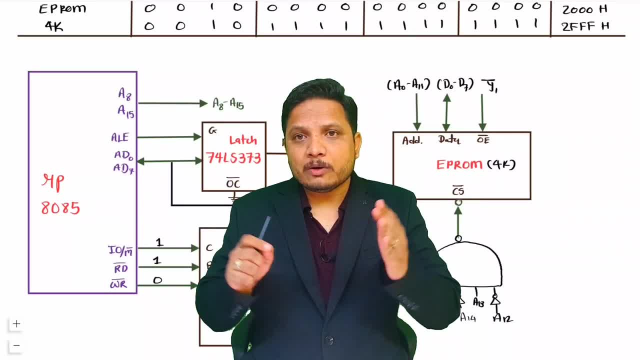 playlist that will ensure that you will be able to interface any complexity of memory interfacing. I hope it is clear to you. thank you so much for watching this video.